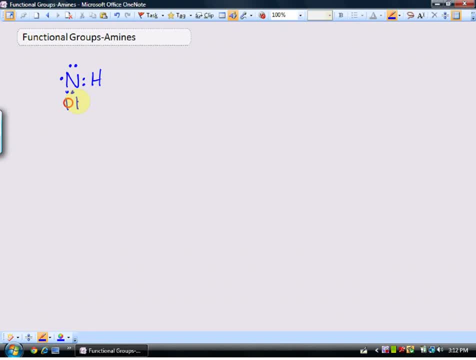 that three hydrogens can come along and each hydrogen shares a pair of electrons with the central nitrogen, and that gives us our simplest nitrogen compound. Now let's talk about a molecule, and I hope everybody knows the name of this very important simple molecule. Its name is ammonia and you've probably all smelled ammonia. It's a very 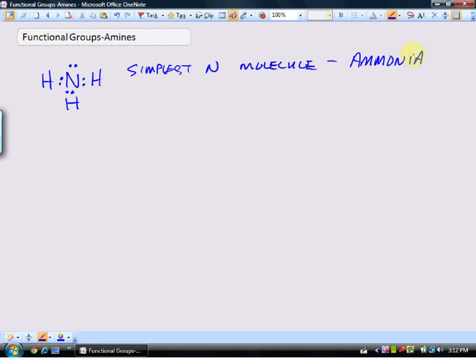 acrid smell Okay, good. So now what we're going to do is: we're going to add, start talking about a new functional group. They're called amines, okay, and notice that they sound a little bit like ammonia, and the focus of an amine is a central nitrogen compound. So we're going to add. 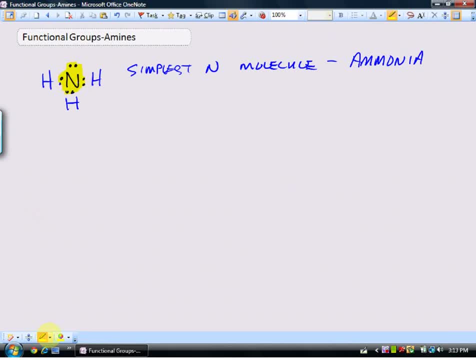 nitrogen and again, nitrogen is always going to have three things attached to it. So in order to make it into an organic molecule, guess what? At least one of those attached groups has to be a carbon group. okay, So we start out, and the simplest amine has a carbon connected to the 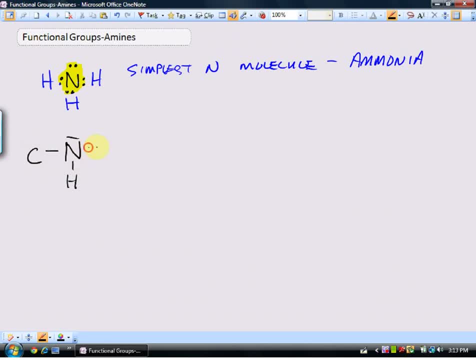 nitrogen, and then the other attachments are hydrogens. okay, So if I fill in all the hydrogens, this would be my simplest Amine and, not surprisingly, that is called methyl amine. I hope that makes sense to you. 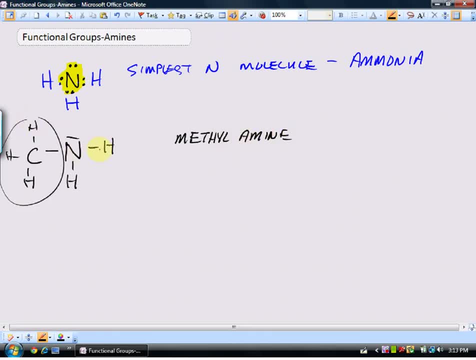 Methyl. we've got a methyl group attached to the nitrogen, and again the focus is the central nitrogen. okay, So that's methyl amine. Now let's add another carbon, and if you think about it now, you've got two possibilities right. So again, we're going to. 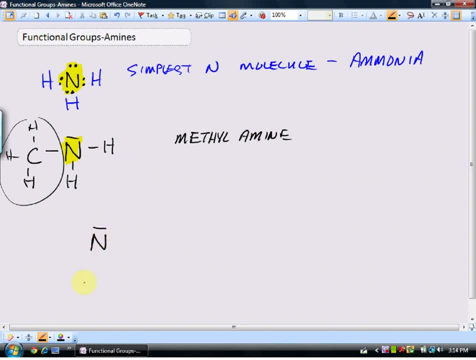 start with our nitrogen, And we've got a carbon already attached on one side. Now we've got two options. We can either attach another carbon here running out of space on the side here, put it in the hydrogens and I bet you everybody can name that. That's ethyl amine. and again, notice, it's real. 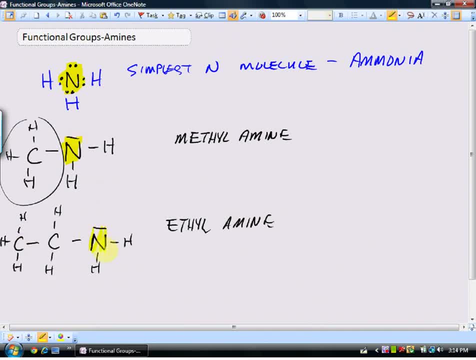 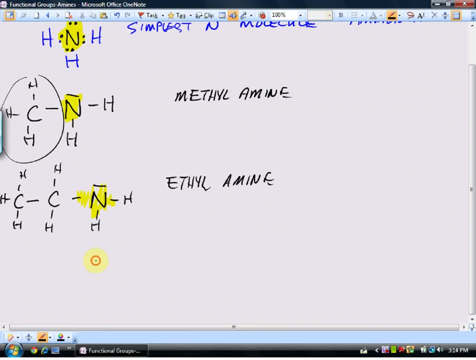 similar to up here. We've got the central nitrogen and attached we've got the carbon group. I hope you've come up with the second possibility. The second possibility is what The second possibility is now. keep my carbon here, but now let's replace one of the hydrogens. 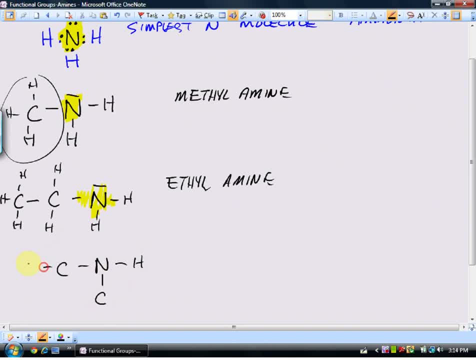 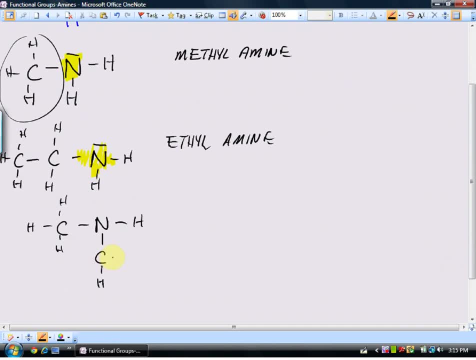 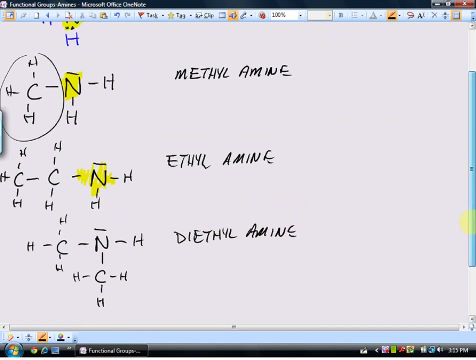 with a carbon And again I put in all of my hydrogens. here I now have a different amine. This is called diethyl amine. Now notice the difference. Up here we had a structure that could be represented by a general formula, R. 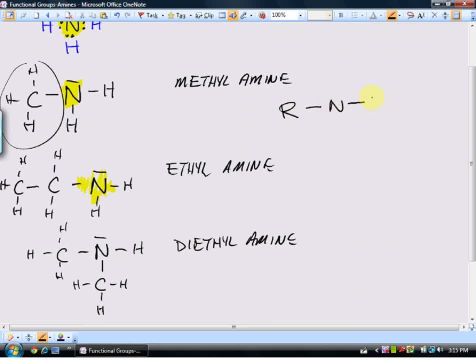 where R is any carbon group connected to a nitrogen, and we had two hydrogens attached. These are called primary amines. Essentially, it means there's only one carbon attached to the nitrogen. We sometimes use that designation for primary. You've probably already discovered what we call these. These are structures that have 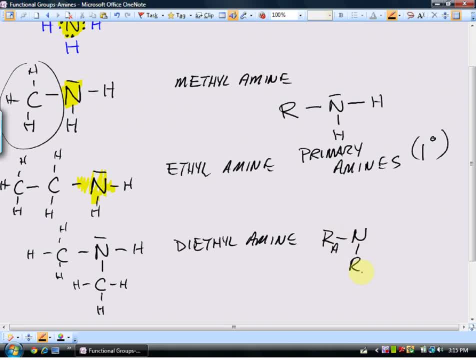 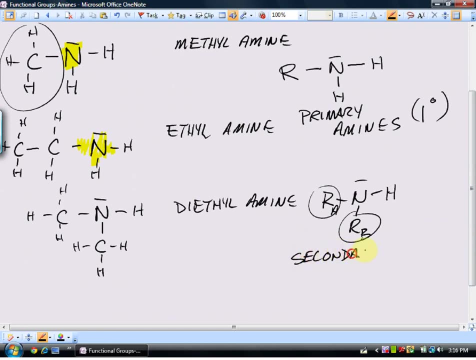 a general formula like this, where there are two carbon groups attached to the central nitrogen and we call those- you guessed it- secondary amines and we use the decimation that as an abbreviation. Alright, So again, secondary amines have. 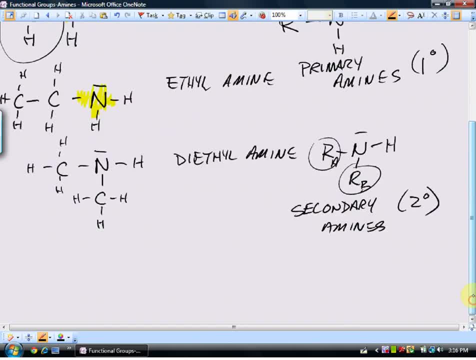 two carbon groups attached. So you know where we're going. next I hope We're going to add another carbon and now we have several possibilities. We could add it to the original chain and keep it a primary amine. We could go and add it to. 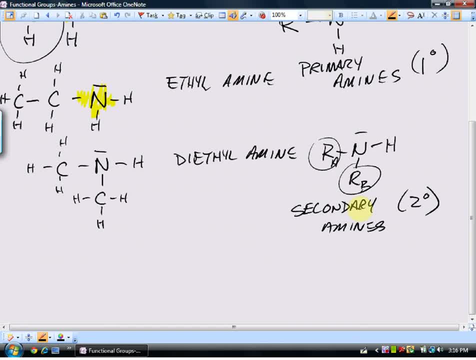 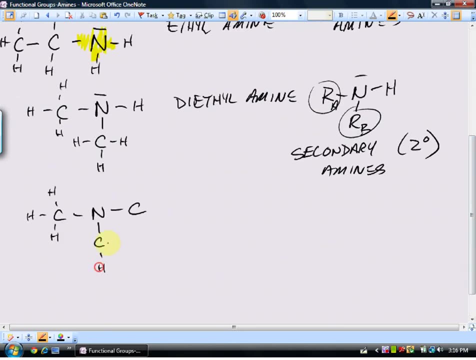 one of the two carbons we have at our secondary amine and keep it a secondary amine. Or we could come along and say: let's replace all of the hydrogens with carbons. Again, I'll take the time to write in all of those hydrogens And we. 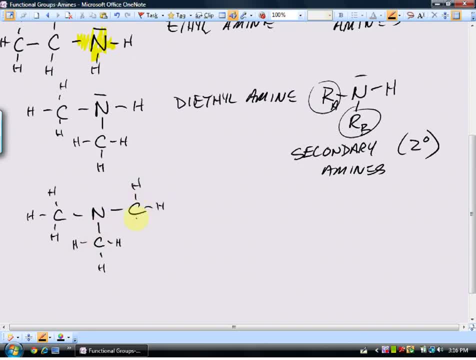 now have no hydrogens connected to the nitrogen and we've completely replaced all of those hydrogens on the nitrogen with carbons, And you're not surprised that. first of all, the name of this is trimethylamine And I hope you know the name. here It's a tertiary.